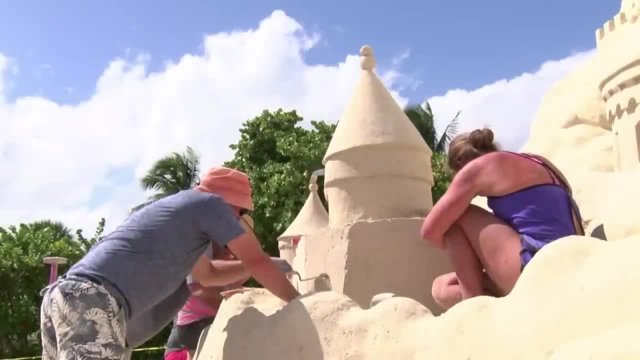 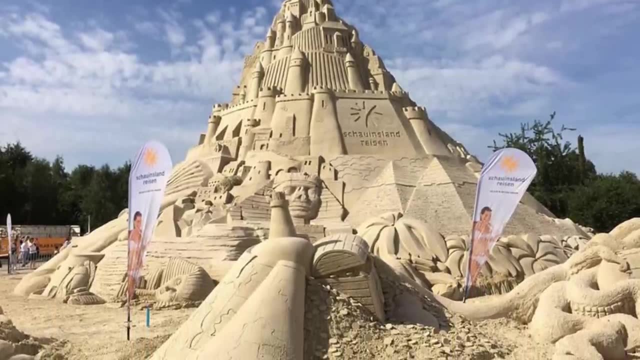 While the point of this sandcastle was to create the tallest sandcastle in the world, the designers still put their all into making it look phenomenal. The castle itself sits on a base of intricately designed sea creatures. that's 85 meters and 3. 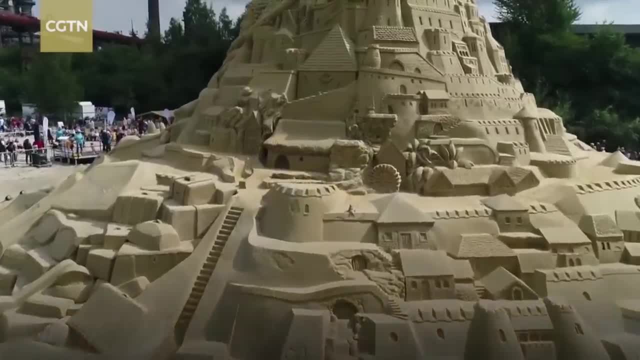 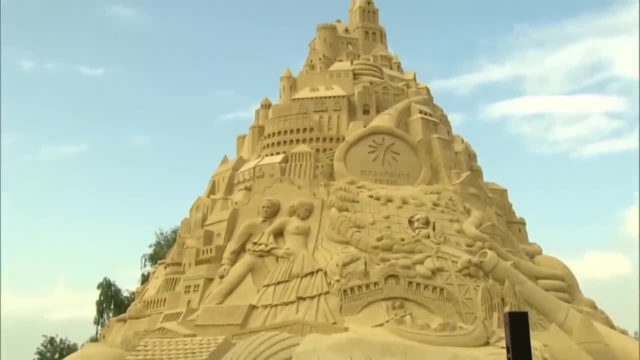 inches wide, which is a set of stairs carved into the side to make it look like an entryway to the main castle above. The bulk of the design is made up of the bottom tier of walls, but as it gets higher the design becomes even more complicated. 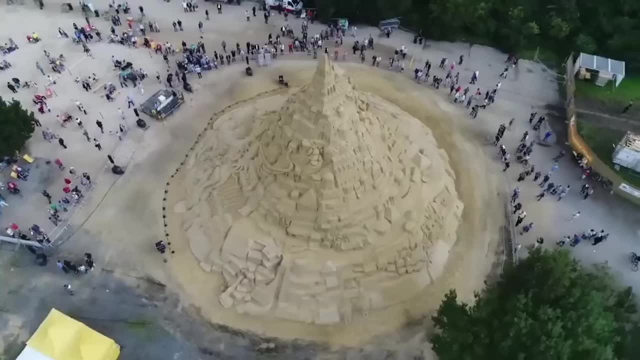 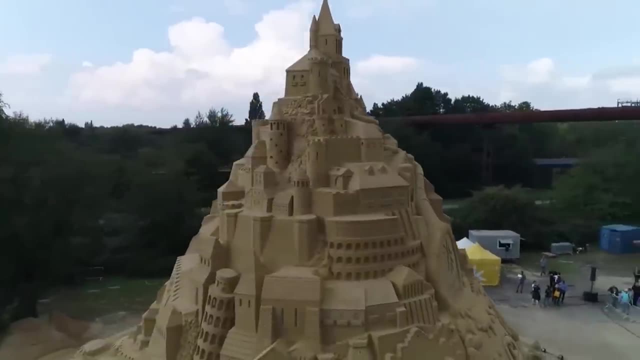 featuring spires and a giant pointed roof right at the top. At 57 feet tall, it's clear to see that the mass of sand is bigger than many of the trees in the surrounding area, and you could just about make out some people walking around it. to give you a, 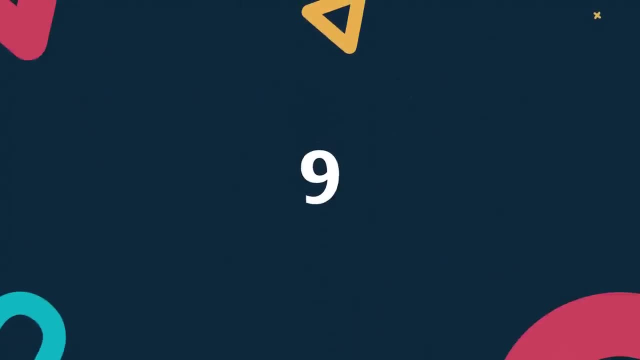 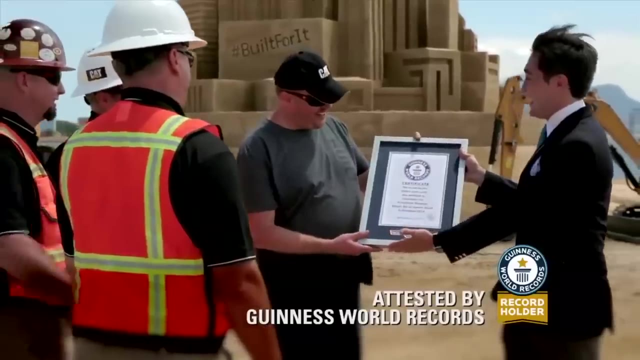 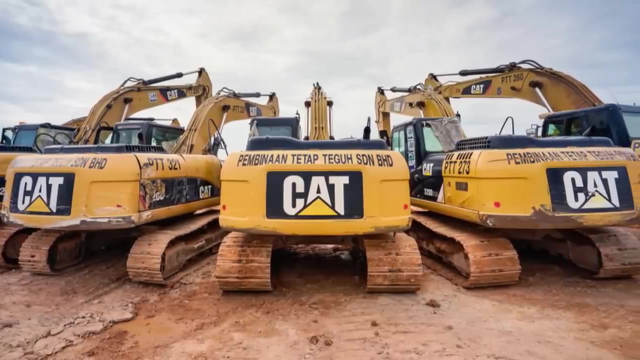 true sense of the colossal creation scale. So before the group of Germans from our last entry on this list came along to steal the Guinness World Record for the world's tallest sandcastle, it was held by the pretty unexpected group of people. In fact, it was a record held by the Cat Company. 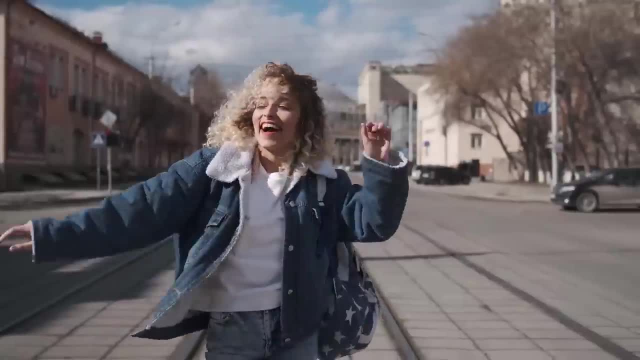 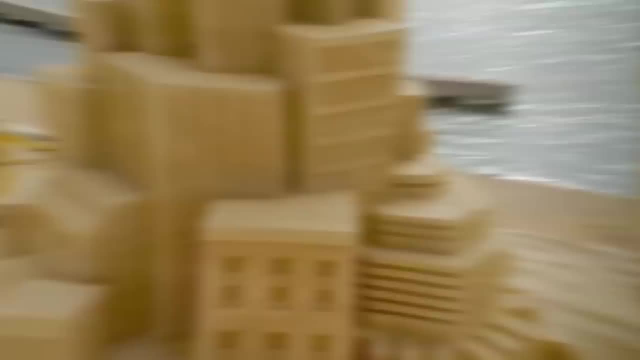 who, you might know, makes heavy-duty construction equipment. That might sound crazy, but when you think about the heavy-duty diggers and lifters that Cat produces, it starts to make a bit more sense. The design itself is much more modern than your typical sandcastle. The ornate spires of 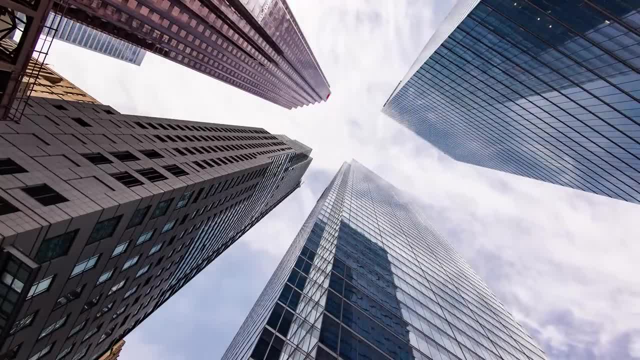 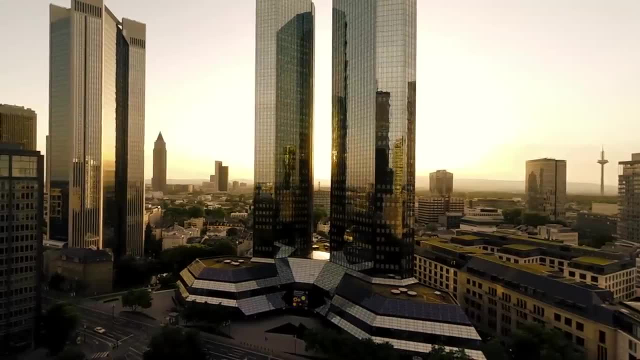 medieval castles have been replaced by tall skyscrapers that tower over everything else nearby. You could argue that the aesthetic of modern-day skyscrapers is much simpler than any other design, but when you realize how thin the design is, you can't help but wonder how thin the 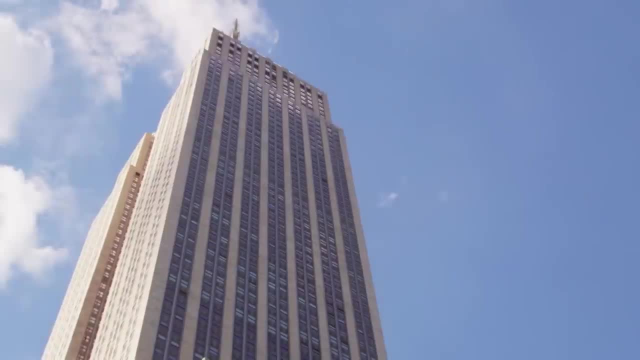 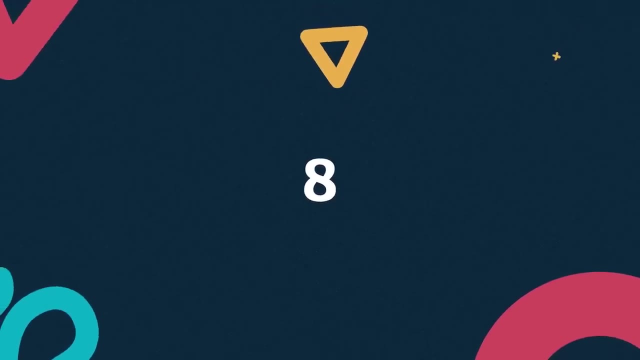 design is You start to realize how much engineering work actually had to go into the design of a structure that could reach so high into the air. The UK doesn't have the best beaches in the world. A lot of them are covered in stone and gravel. 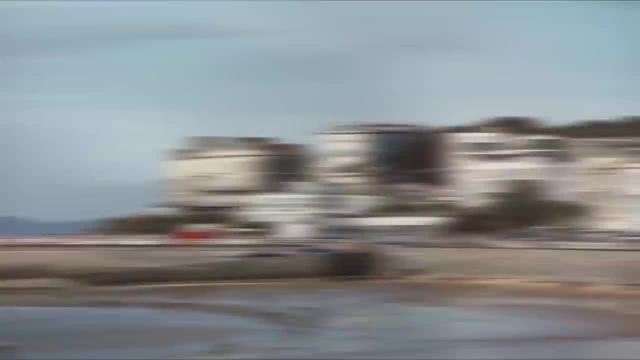 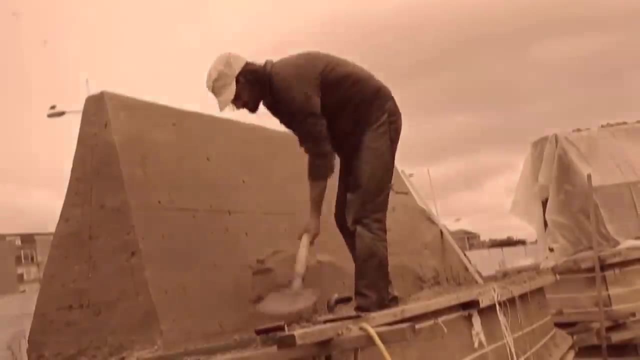 but some are perfect for creating sandcastles. One of those beaches is Weston-super-Mare, and it's home to a yearly sand sculpture festival, where some of the coolest sandcastles in the world are built. The festival has been running ever since 2006,. with each year 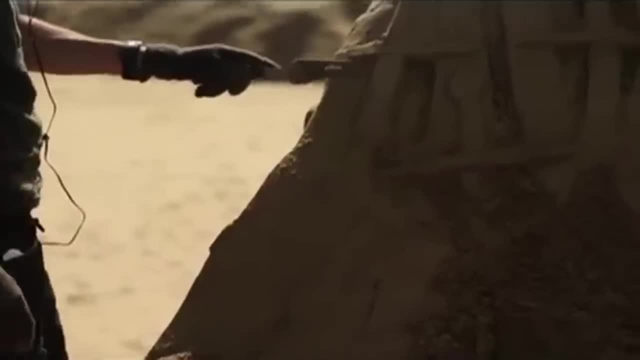 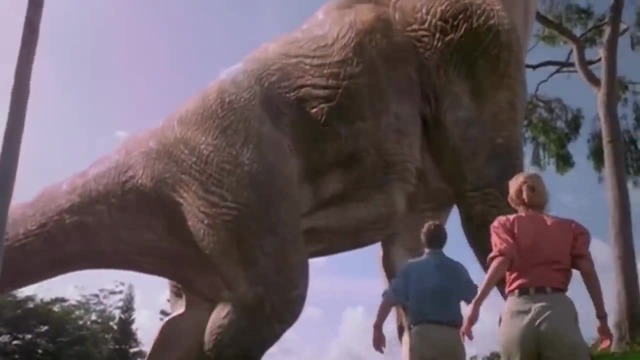 following a special theme In 2019, the theme was What If? where the sand sculptors had to design their sandcastles around a question, Some of the examples being what if the dinosaurs returned? or what if you were the only person on earth, While all of the sculptures at the festival. 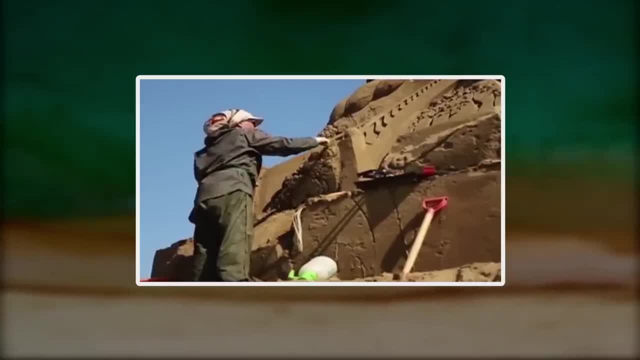 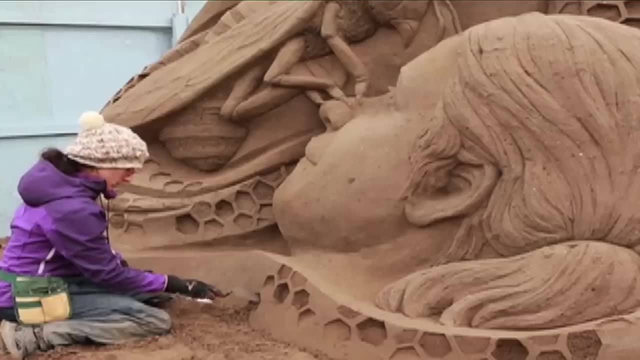 are cool in one way or another. the one we liked the most this year is the sculpture of a chef. He seems to be deep in thought, wondering what to do with the chicken in the sand and the potatoes off to the side. I guess the question that the sculptors were asking. 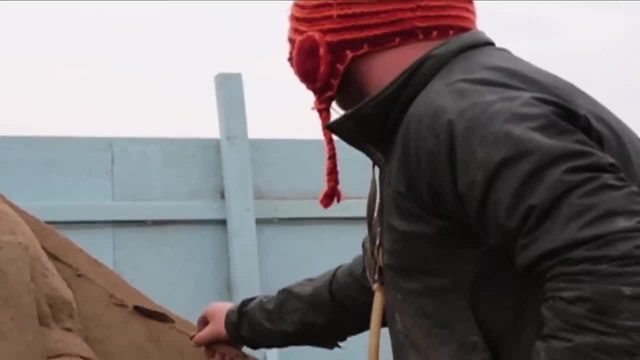 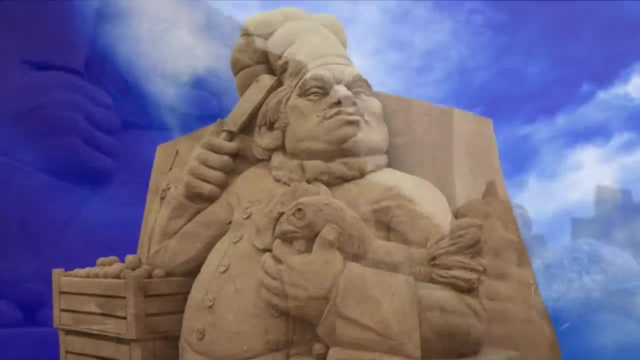 when they built this sandcastle was: what if we had chicken for dinner or something like that? The amount of detail that went into creating each element of the sandcastle is pretty insane, from the ruffles of the chicken's feathers to the look of deep thought on the chef's face. 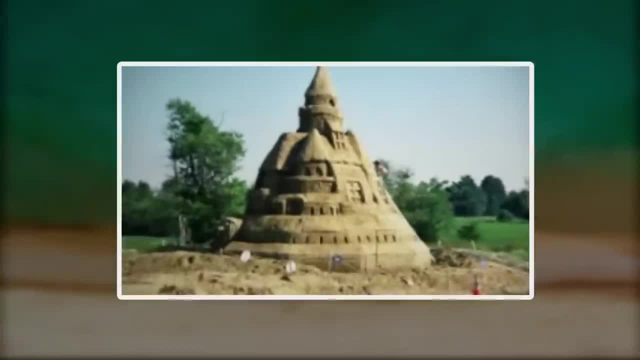 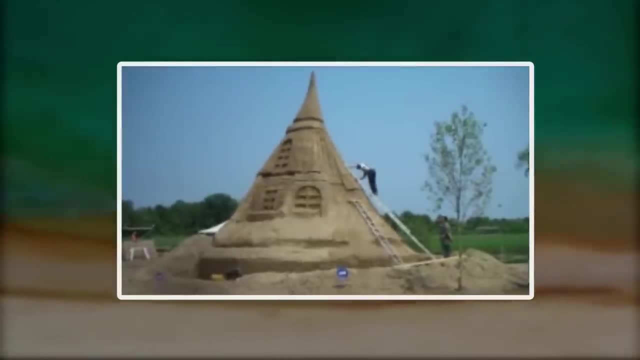 Ed Jarrett is a bit of a legend in the sandcastle world. The first time he broke the world record for the world's tallest sandcastle was in 2003,, where he built a castle that was 29 feet and 3 inches tall in Maine. He followed that up a few years later with another castle. 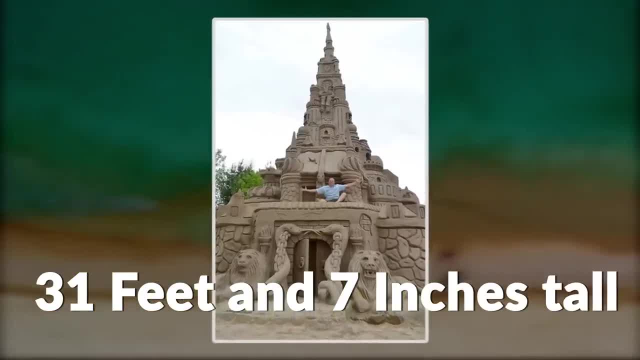 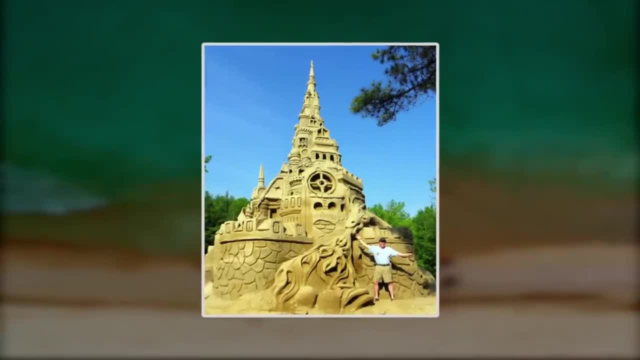 once again built in Maine that was 31 feet and 7 inches tall. All of that led to his final build in 2011,, where he built a sandcastle that eclipsed the others at 38 feet and .75 inches tall in Farmington. 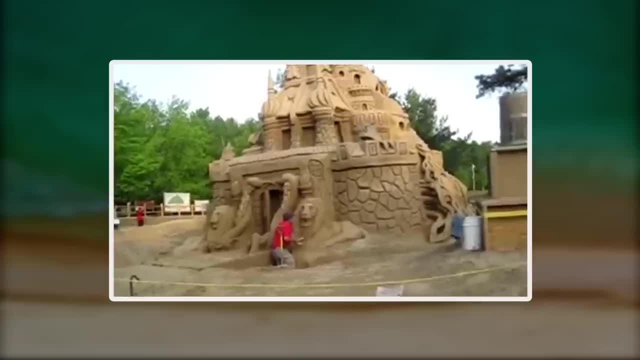 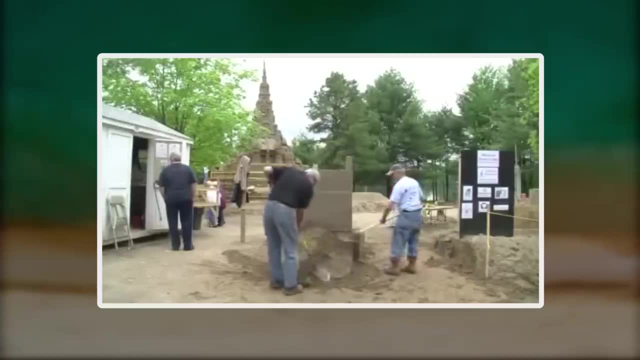 The castle is a giant structure with immense detail, from lions and fire-breathing dragons guarding the walls at the bottom to intricate castle spires at the top. The sandcastle really focuses on the medieval aesthetic and looks really impressive as it towers above some of the nearby trees. 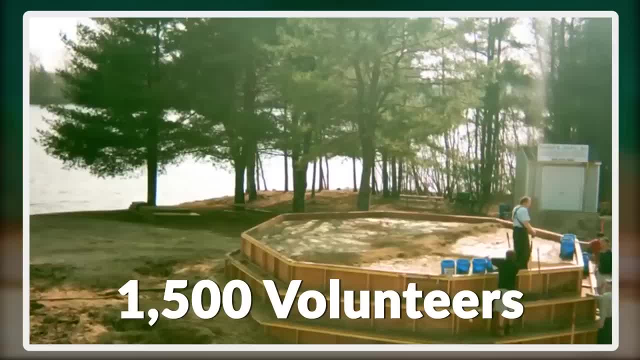 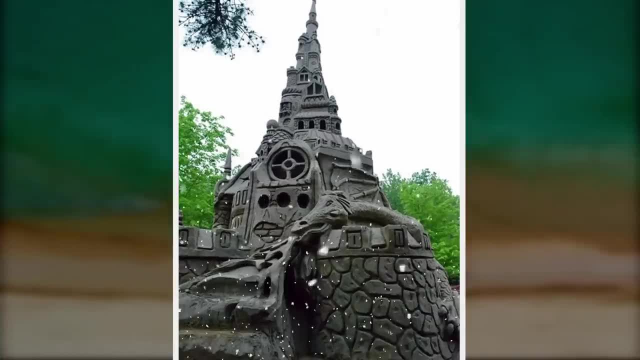 The build took the work of 15 artists and around 1500 volunteers to complete over 2500 hours. It wasn't easy. the weather tried to stop them at every turn. They had to deal with snow and even a thunderstorm the night before the final measurement of the castle. 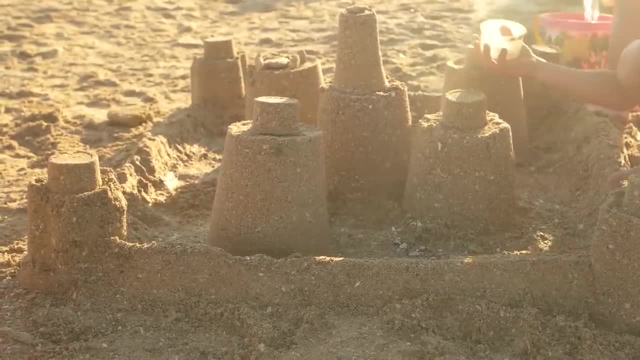 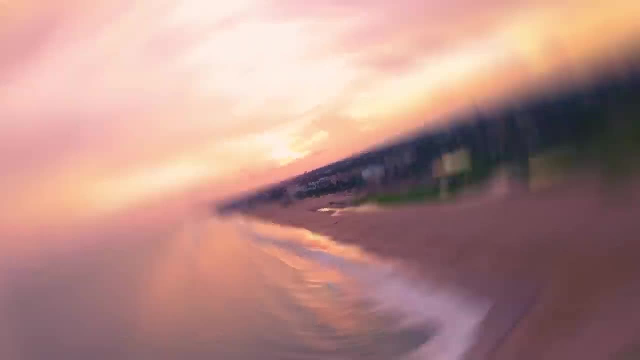 The battle over the world's tallest sandcastle is one that never ends, and for a brief period in 2017, the Guinness Book of World Records award went to a castle that had been built in India, at Puri Beach. The design stretches 48 feet into the sky and is covered in sand, doves, turrets and 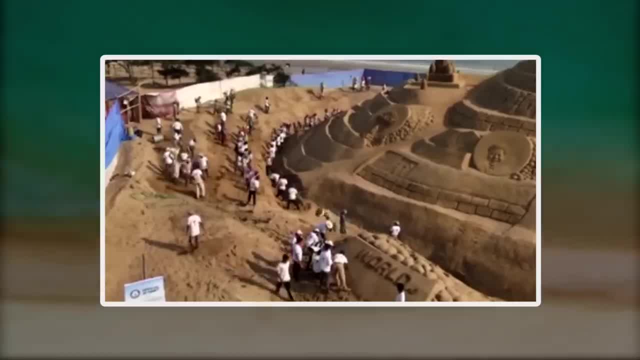 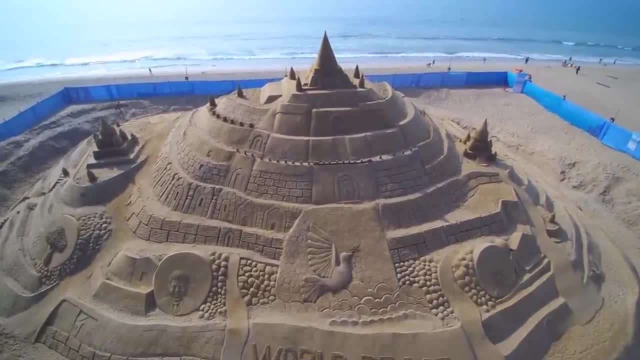 a gigantic portrait of- you guessed it- Gandhi. The sandcastle was constructed by a group from the Sudarshan Sand Art Institute over the course of four days. The design of the sandcastle honestly seems like it could have gone even taller, Like instead of continuing to go upward in. 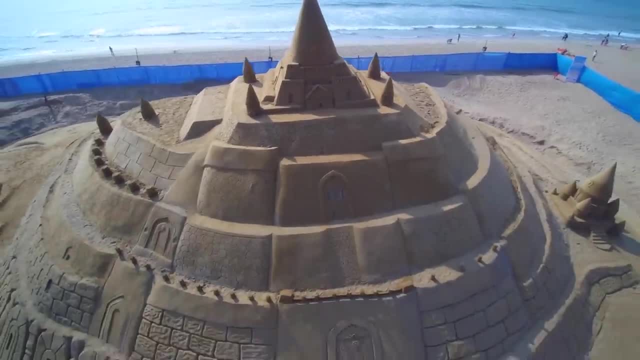 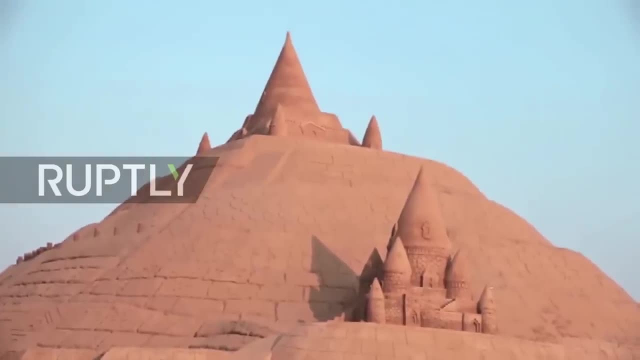 tiers, as they have been doing. pretty much like the whole design, it's topped off by a slightly smaller, detailed castle. Either way, when people stand close to the design, it looks more like a sand mountain than a sandcastle, so it is absolutely enormous. 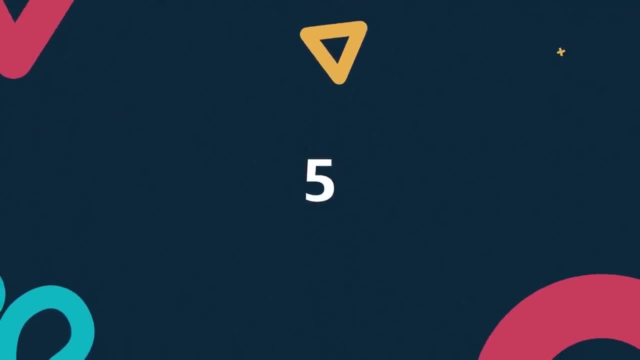 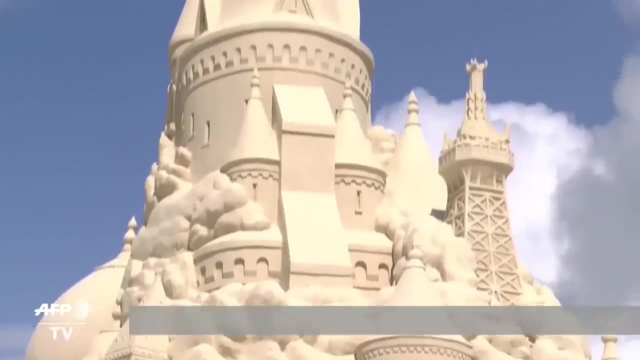 5. Sand Mountain. If you head to Virginia Key Park, then you're going to come across another of the world's tallest sandcastles. The castle is based around some of the world's most important and symbolic buildings, including the Taj Mahal from India, the Leaning Tower of Pisa from Italy. 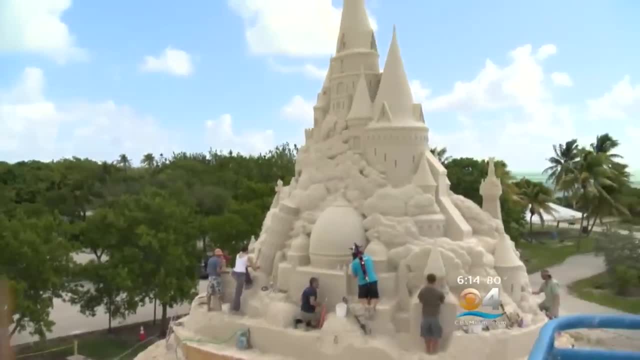 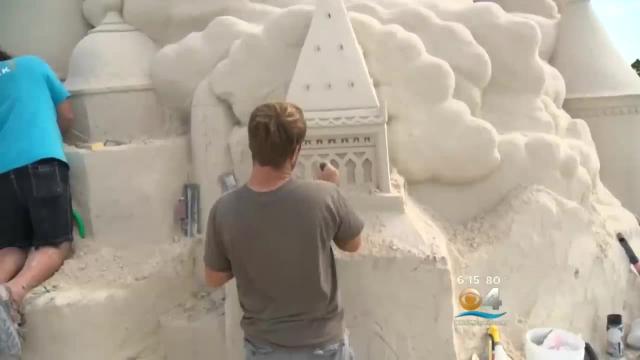 and the Eiffel Tower from Paris. The strange thing about this build is that there are no signs around the construction to show off who built the thing. so unless you were to research it further, you would never know that the only reason this immense sandcastle exists. 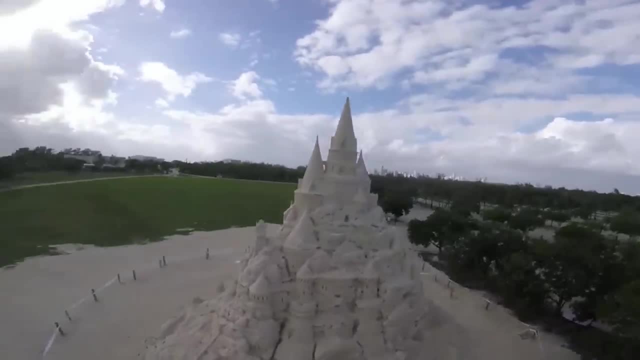 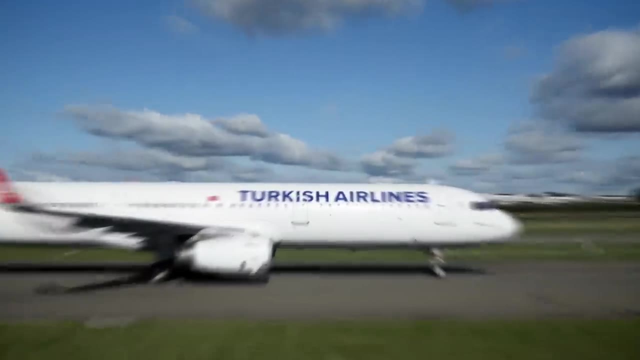 is because of Turkish Airlines. Yeah, the airline sponsored the award-winning sandcastle creator, Ted, to build the sandcastle to act as a publicity stunt for a New Miami to Istanbul flight. The end structure stood at 45 feet and 10 inches tall and was crafted from over 1,800 tons of sand. 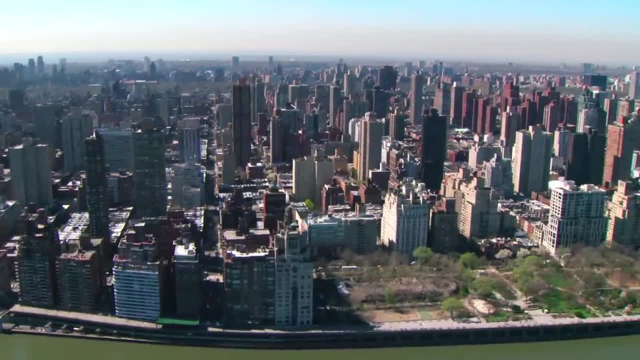 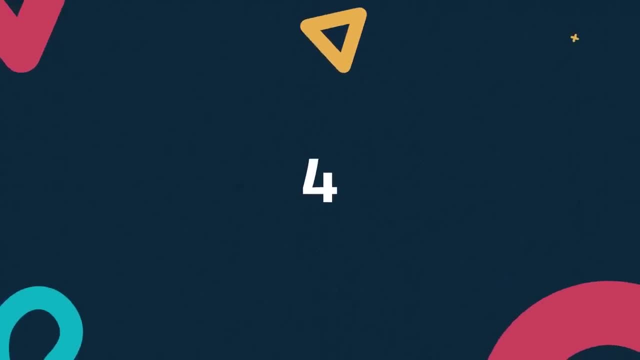 by a team of 19 artists. Almost every country and major building in the world is represented in the piece carved out of the sand in deep detail. In 2007,, the world's tallest sandcastle could be found at Myrtle Beach in South Carolina. 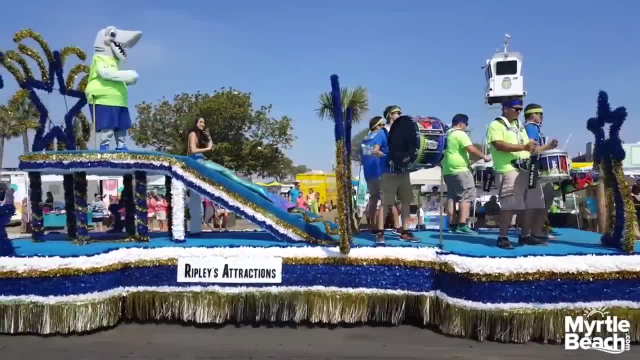 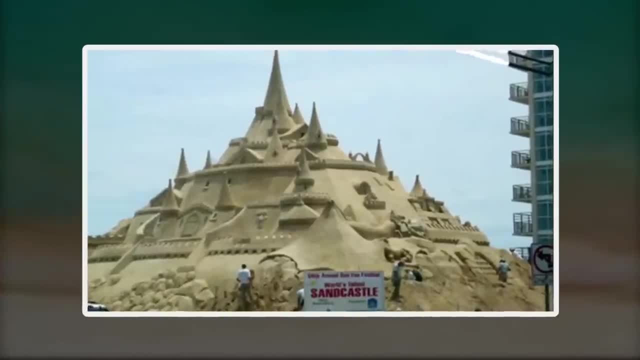 and had been put together a week before the annual Sun Fun Festival. This sandcastle design is one that takes a more traditional route. It's literally one giant castle. There are multiple pointed spires across the design, with one large central spire in the 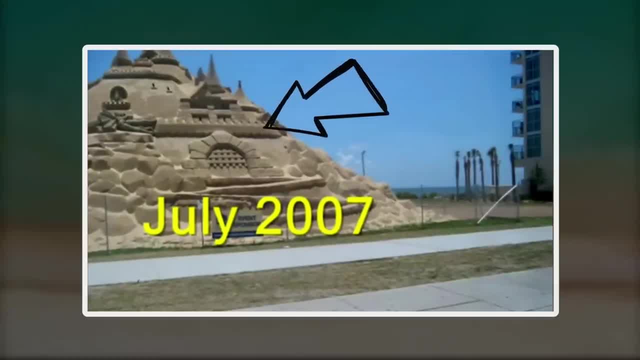 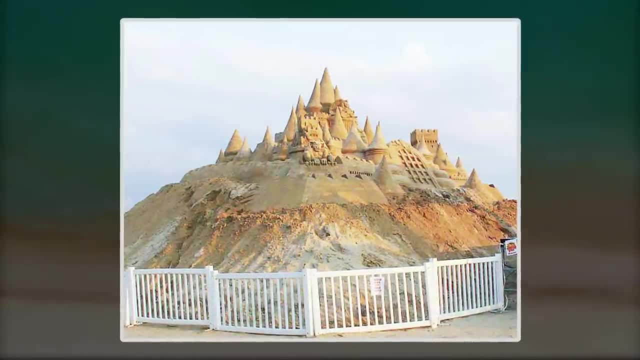 middle to make up the height. At the bottom of the castle there are big gates and there's even a sand dragon carved into the side of the design. After being completed, the base of this immense sandcastle was 60 feet wide and the peak reached up to 35 feet into the air. It took the sandcastle 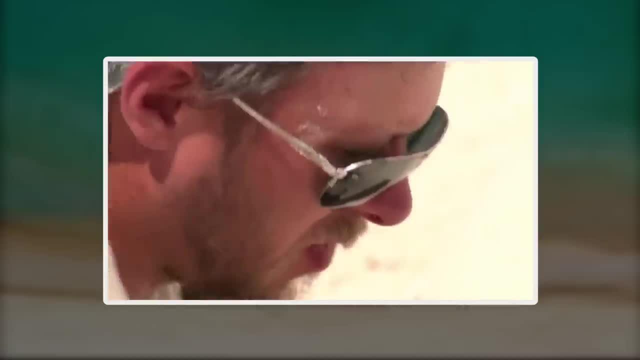 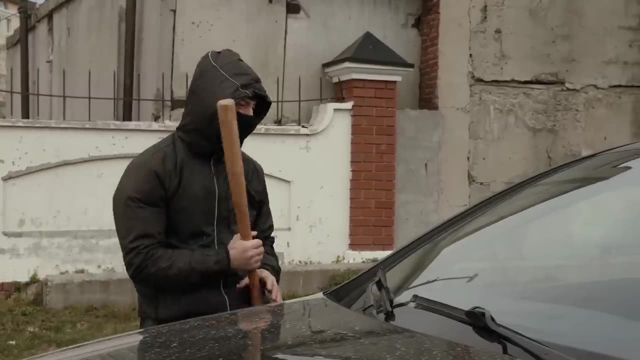 sculptor's 130 dump truck, loads of sand and just over a week of construction to complete. Even crazier, over the course of construction, the sandcastle was damaged by vandals, as well as wind and rain from Tropical Storm Barry, but it was still able to break the whole world. 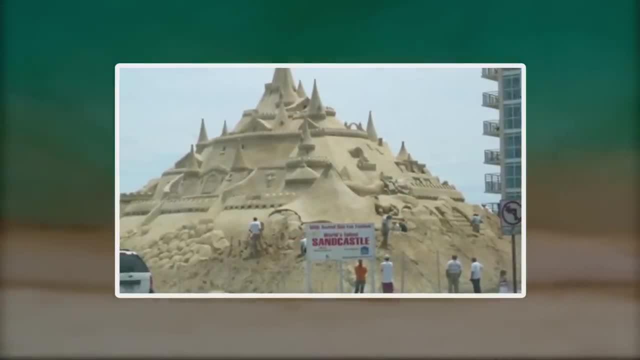 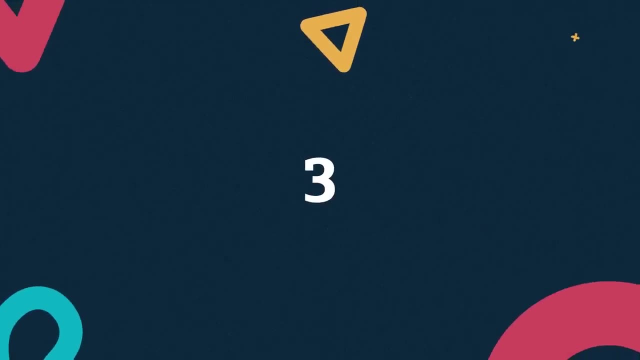 record. The castle was built on the site of a building that had just been knocked down and actually had to be taken down itself shortly after, so the new building work could begin at the site. The city of South Padre Island loves sandcastles so much that they have an annual 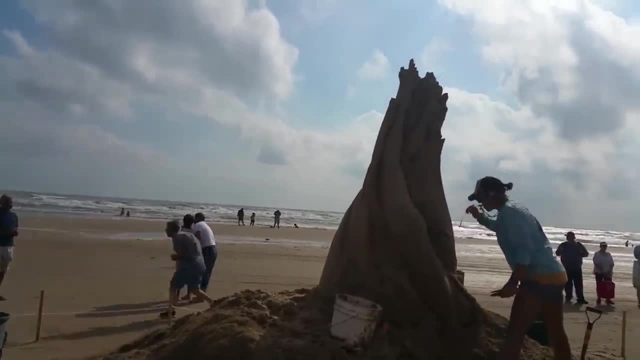 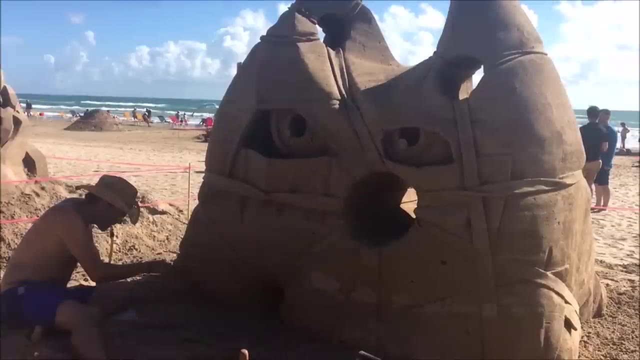 event dedicated to incredible sandcastle creations. They call it the Sandcastle Days. It was started 32 years ago to demonstrate not just the sand sculpting abilities of those who live in the area, but to highlight the importance of protecting the coastal shores of the states. 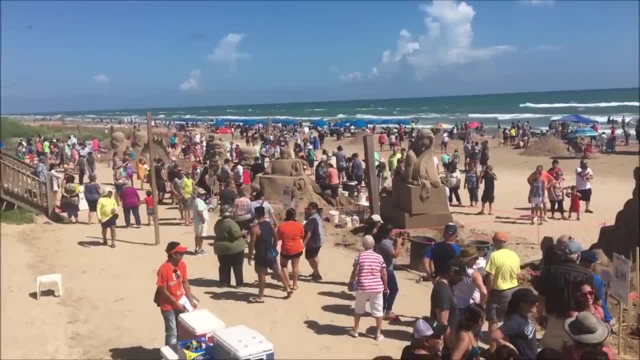 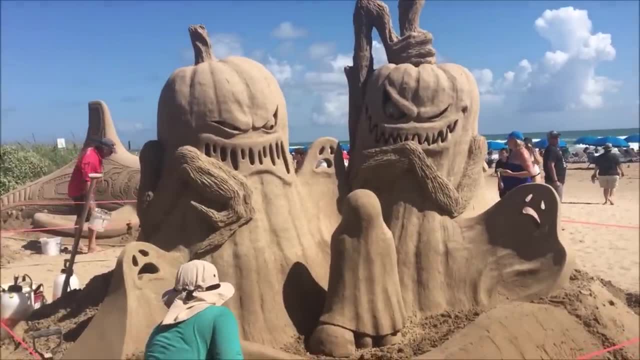 The event is free to attend and has grown from a local celebration of sand sculpting to a qualifying event of the Sand Sculpting World Championships. Because of that, the sand sculptures in this area are some of the biggest and best in the world and have a quality that 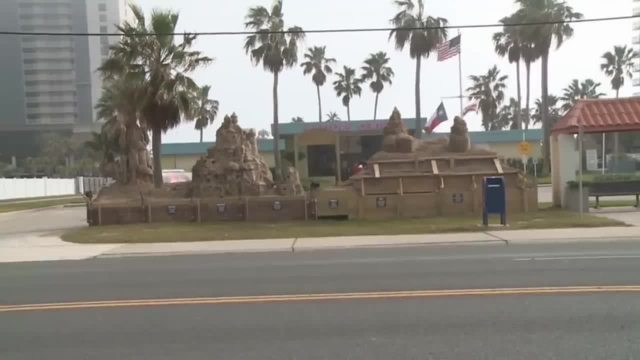 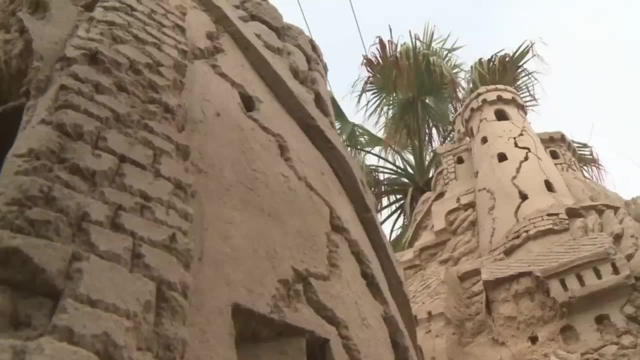 is almost unrivaled by anywhere else. One of the best sand sculptures in the area is a permanent sculpture that was created by an Australian named Andy Hancock. He started life as a woodcarver but switched over to sand when he realized how interesting it was to work with as a material. 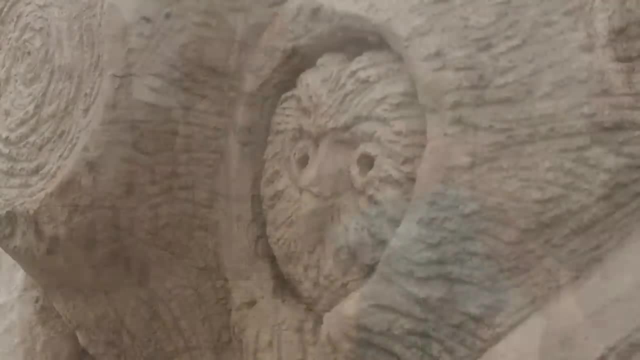 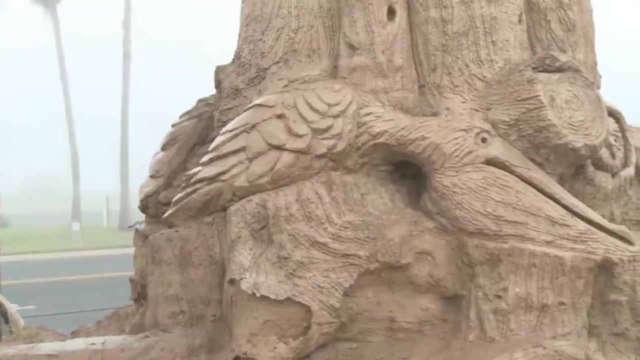 His South Padre sand sculpture is an incredibly detailed castle, and each part of the castle has its own story that Andy developed. For example, the dragon is built into the stone wall and, according to Andy, it's because the dragon attacked the castle and the wizard turned it to. 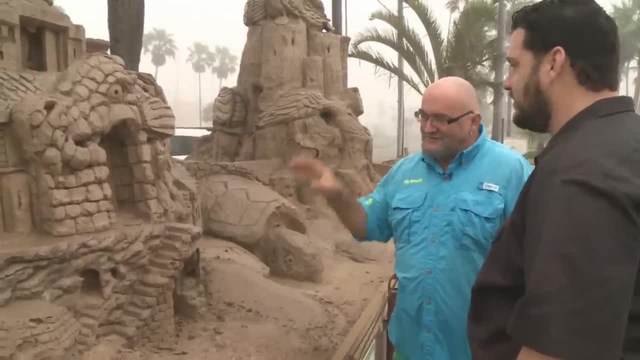 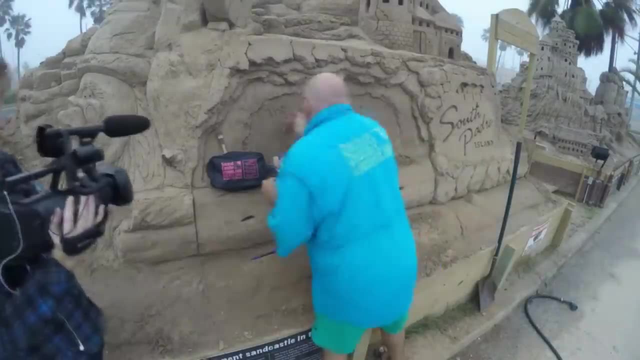 stone. To make the sandcastle permanent, Andy has coated the structure in a thin layer of glue which helps it stay standing strong through all weather conditions. But Andy is still working on his giant structure even to this day, adding more and more to make South Padre's biggest ever sandcastle even bigger and better. 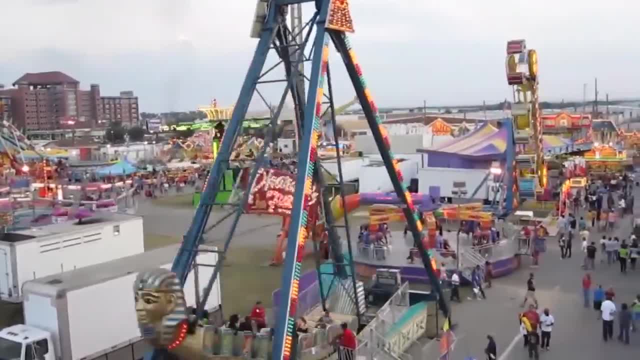 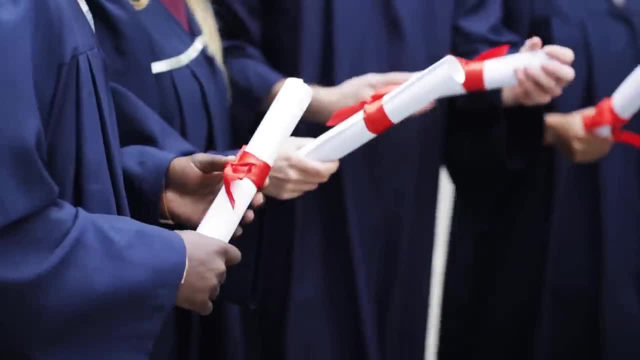 The South Carolina State Fair is a yearly 12-day long event held in Columbia which raises money and donates millions of dollars in scholarships for students in South Carolina. Every year they award 50 scholarships to high school students in the states and part of that money is raised by the sand sculpture exhibit they have there every. 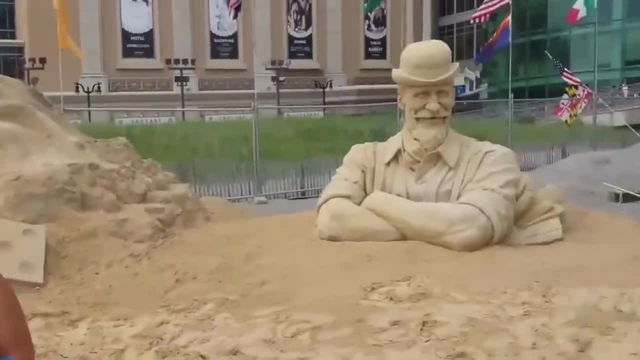 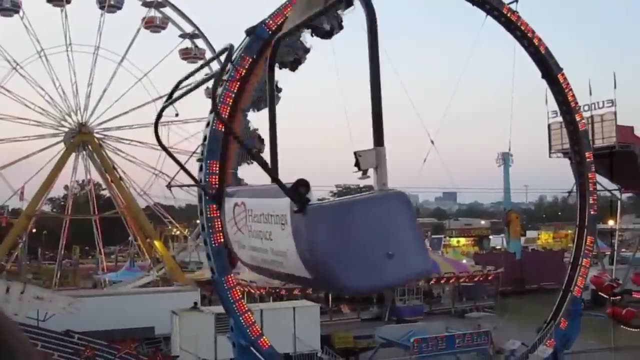 single year Over the course of the fair. the sandcastle sculptors from the event, who have over 10 World Sand Sculpting Championships under their belt, create incredible sand sculptures for people to look at During the 2013 South Carolina State Fair. this sand sculpture has a giant castle. 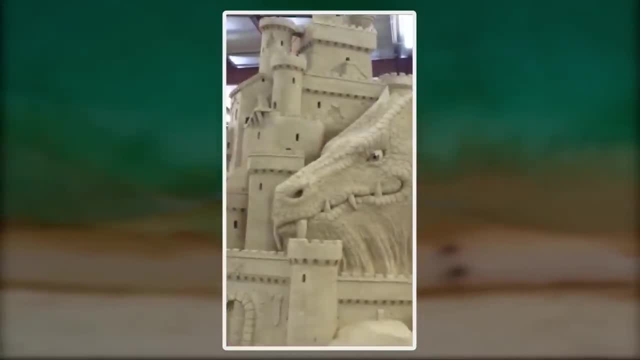 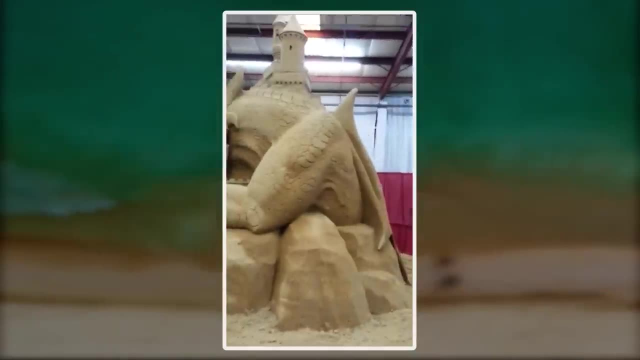 which was being attacked by an even bigger dragon. The sculpture had a level of detail that was far beyond what most sand sculptures have, even outlining the ripples and contours of the giant dragon's muscles and skin. The giant dragon had its neck and hand wrapped around one side of